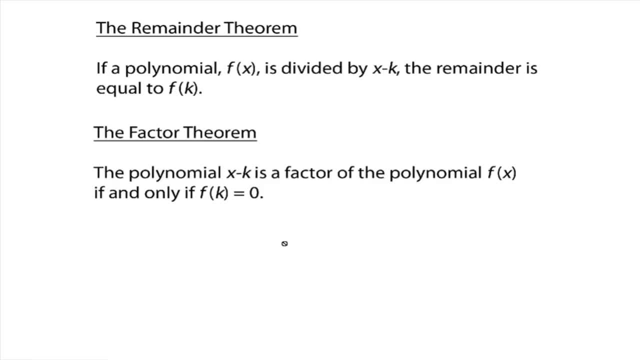 because that's what the remainder theorem was saying here. then x minus k would be a factor. Okay again, if you're still not, if you're still not sure, if you're still not sure, if you're still a little shaky, hold on. 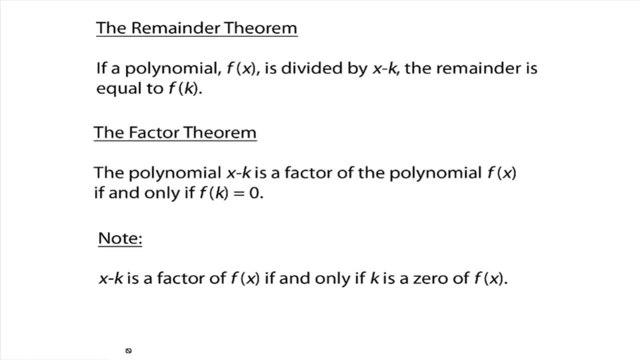 Okay, so a little note Alright: x minus k is a factor of f of x if, and only if, k is a zero of f of x. And remember what it means to be a zero of a function. A zero of a function is any number that, when you evaluate it into your function, 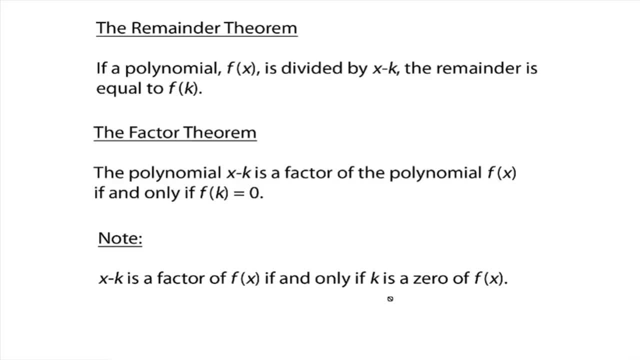 the value of the function turns out to be zero. Okay, that's what this thing right up here in the factor theorem is saying. If you evaluate your function f at some k value, and then that's what you get, and that function value goes to zero. 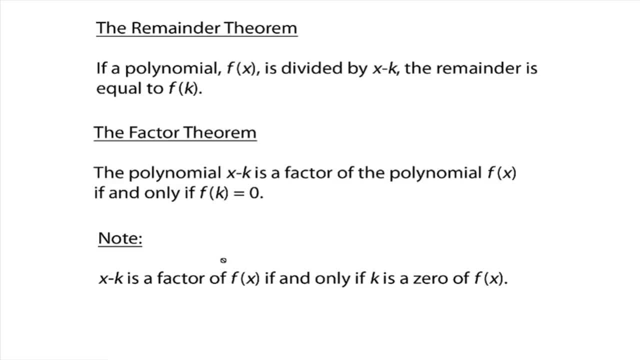 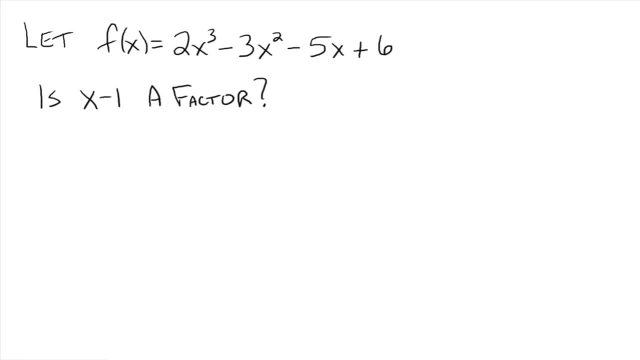 then x minus that k value is a factor of your polynomial Alright, Alright, so enough of the theory stuff. Let's do an example. Alright, let f of x be 2x cubed minus 3x squared minus 5x plus 6.. 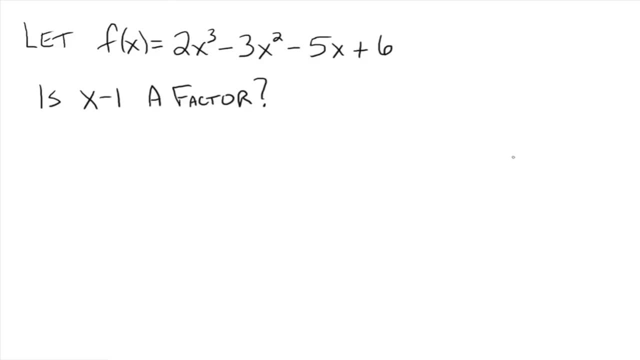 So the question is: is x minus 1 a factor? Well, one way to do it would be to find f of 1.. Because your k value here is 1.. Okay, well, what's f of 1?? Alright, so you plug 1 in for all the x's. 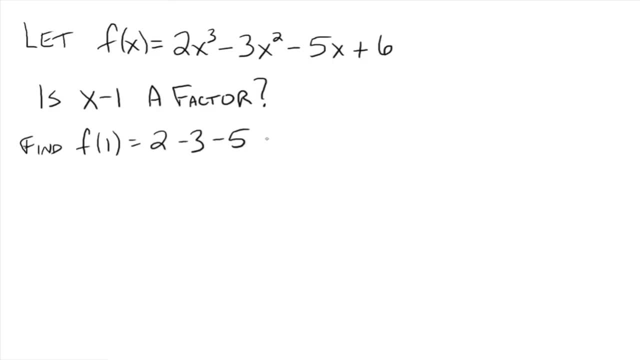 and you get 2 minus 3 minus 5 plus 6, and that all goes to what Everybody get, that It all goes to zero. Alright, so because f of 1 is equal to zero, then x minus 1 is a factor of this polynomial f of x up here. 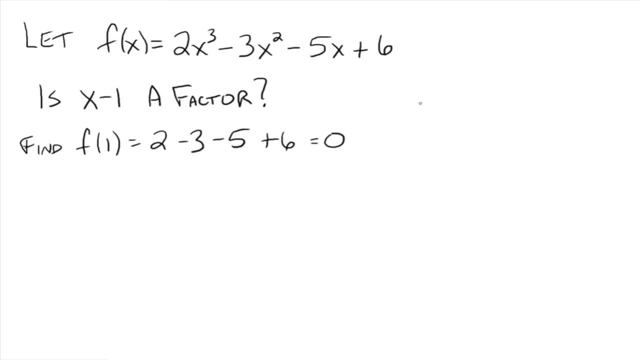 Alright, so that's f of 1.. Fine and dandy, but we can actually do something else that would be even more useful. Alright, so the other thing we can do is we can do the division. We can divide x minus 1 into f of x here. 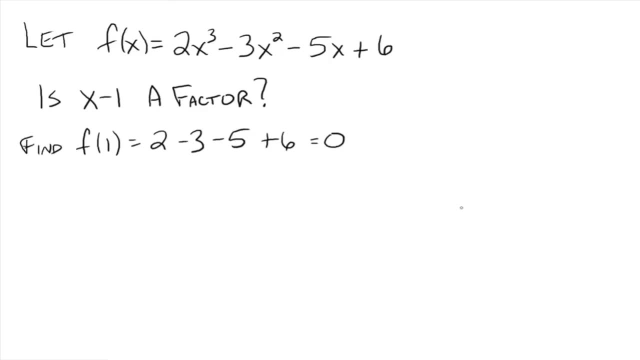 and if the remainder turns out to be zero, then x minus 1 is a factor. Okay, And we're going to use synthetic division because well we can. It's x minus a number here, So let's put 1 inside our little half box. 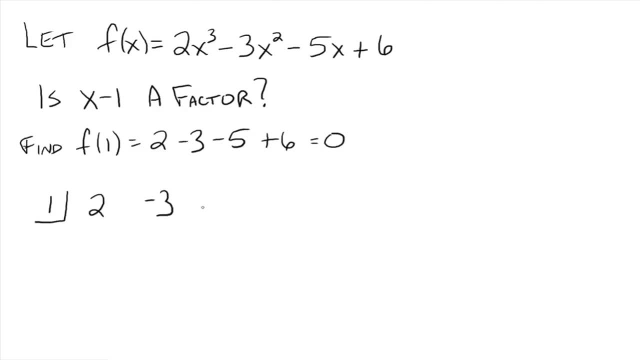 and out to the right. here we have 2, negative, 3, negative 5 and 6.. Skip a line, draw a line, Bring the 2 down and go 1 times. 2 is 2.. It's negative 1, negative 1, negative 6.. 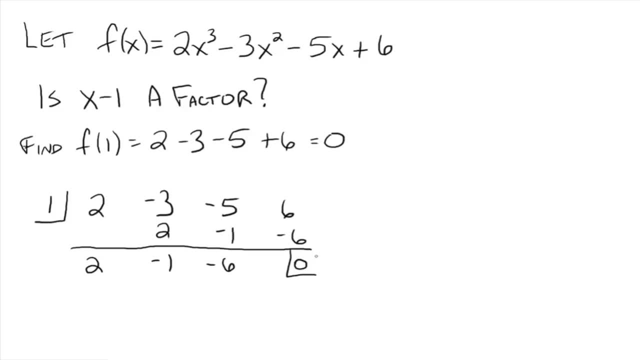 Negative 6 is zero. Okay, And we got zero. Just like the remainder theorem said, we would get That- the remainder. if you divide x minus 1 into f of x here, then the remainder zero is the same thing as if you were to evaluate the original function. 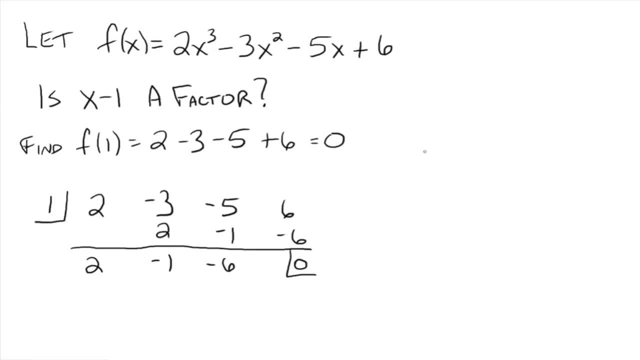 at that point That k value 1.. And they are the same. Everybody see that. Okay, Now with the factor theorem. we know that x minus 1 has to be a factor. So if you'd like to just say yes, we're excited, yay. 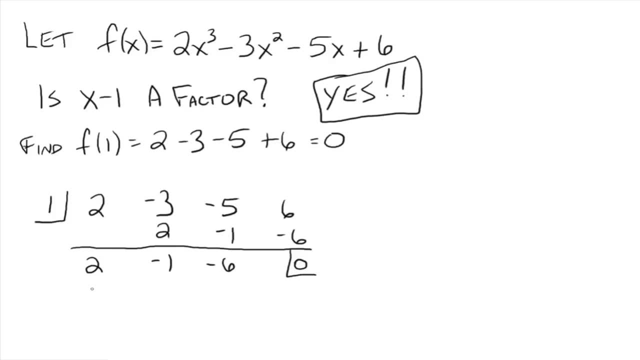 Okay, it's a factor, And so then your quotient down here would be 2x squared. Remember you started with x cubed, 2x cubed. so this is cubed. So this is squared 1 degree less. 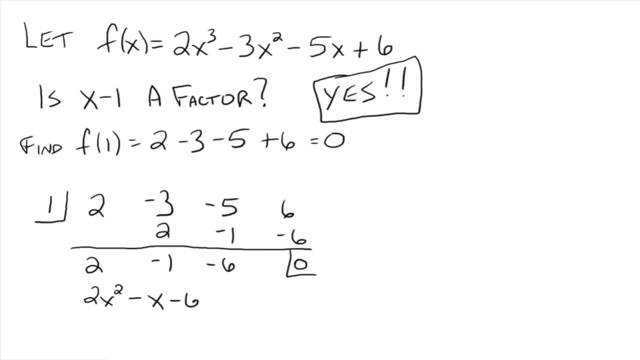 and then you go in descending order. So minus x minus 6.. All right, So really what we have now is f of x has been factored into x minus 1 times 2x, squared minus x minus 6.. Everybody see that. 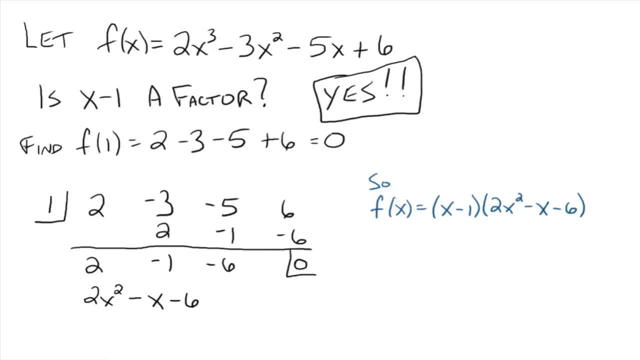 If you take this quotient and multiply it times x minus 1, the divisor there, you're going to get back your f of x, 2x cubed minus 5x plus 6.. But now let me ask you: does 2x squared minus x minus 6 factor? 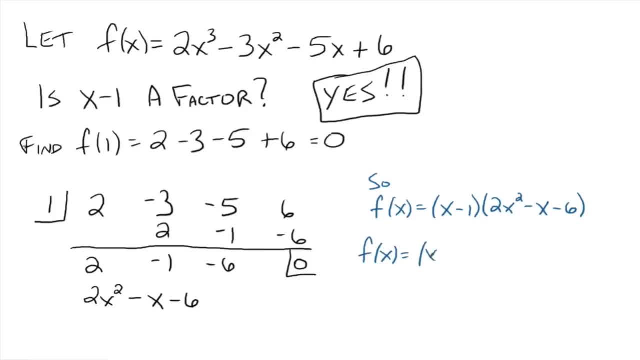 Okay, Yes, it does. So we have x minus 1.. Then 2x squared minus x minus 6 factors into 2x plus 3 times x minus 2.. Everybody see that, Okay, So I'm writing it down here in this, completely factored in form. 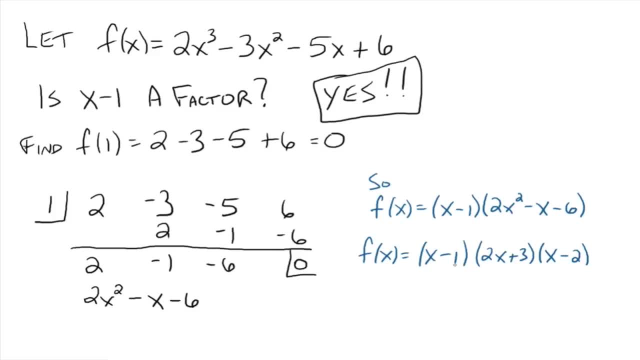 Okay, So I'm writing it down here in this, completely factored in form. Okay, So I'm writing it down here in this, completely factored in form. We've just taken a third-degree polynomial and factored it into a product of three factors. 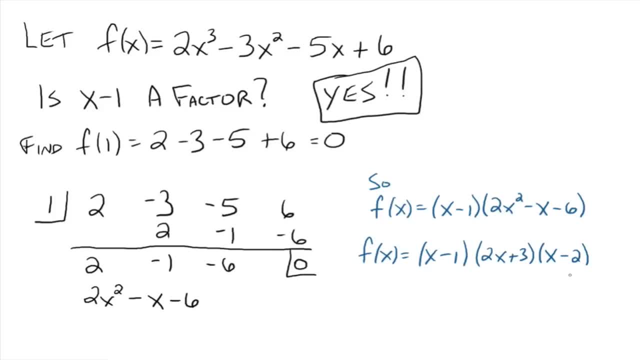 And these three factors down here. look at each part: x minus 1,, 2x plus 3, and x minus 2, those are all linear expressions. Everybody see that, In fact, all three of these things down here are called linear factors. 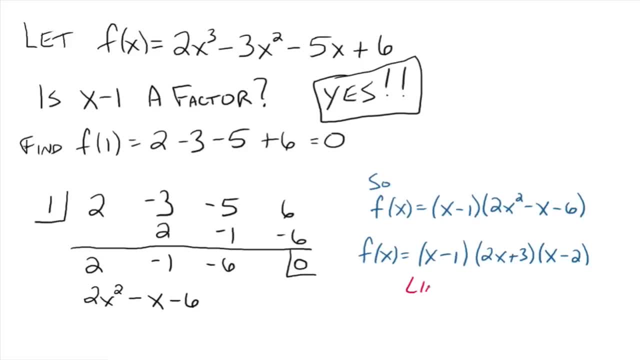 I'm going to write that up. We've got linear factors. Okay, We like to write if we can. we like to write our polynomials as a product of linear factors. One reason why is now we can read off all the zeros. 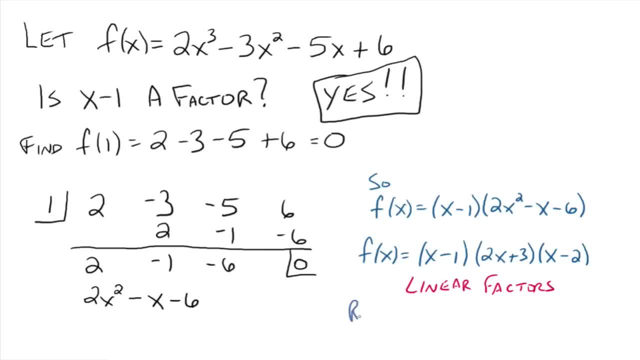 Right, Everybody see that. So we've got real zeros. So we have real zeros. Okay. Real zeros are what makes the y value zero. Okay, so everybody see that if x was one, it'd make the y value zero. 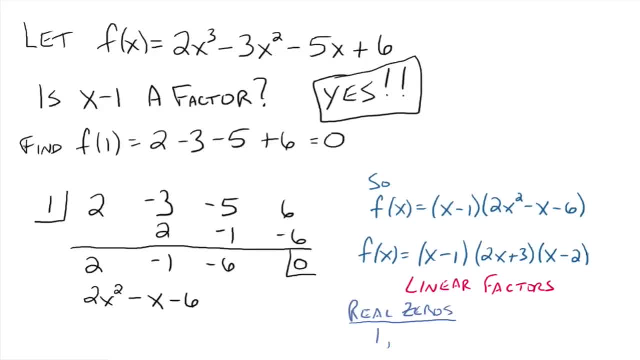 We already figured that out over here. One, okay. If x is two, everybody see that This would go to zero. so the whole thing would go to zero. And if x is, what's this? one Negative, three halves right. 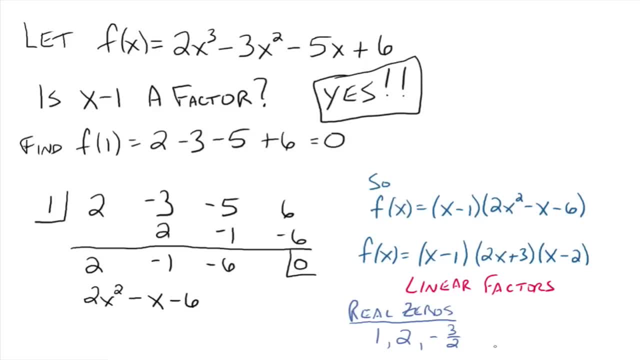 If you set each one of these factors equal to zero, you'll get these three numbers down here, And these three numbers are called the real zeros of our function. And all that means is if you take any one of these three numbers and plug them in for x up here. 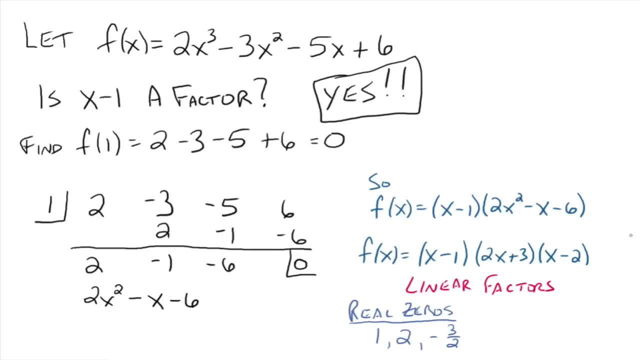 then the y value goes to zero. Great. Now what does that mean graphically? That's right. This is where we hit the x-axis, right? If we were to graph this function, we would hit the x-axis at one comma zero. 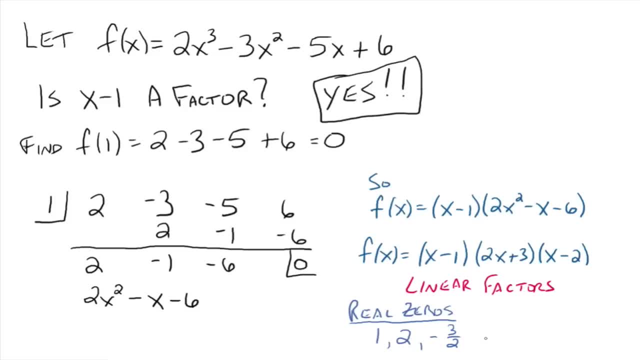 two comma zero and negative three halves comma zero. Follow me. Okay, so this process is called linear factorization. You're trying to write this polynomial, this original polynomial, as a product of linear factors, And one way to do that is do synthetic division. 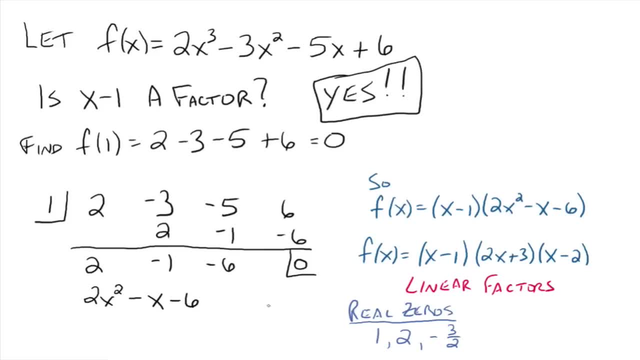 get a remainder of that zero and then take your quotient and then you keep doing the synthetic division for as long as you need to, But as soon as you get your quotient down to a quadratic, well then you can try to factor it and see what happens. 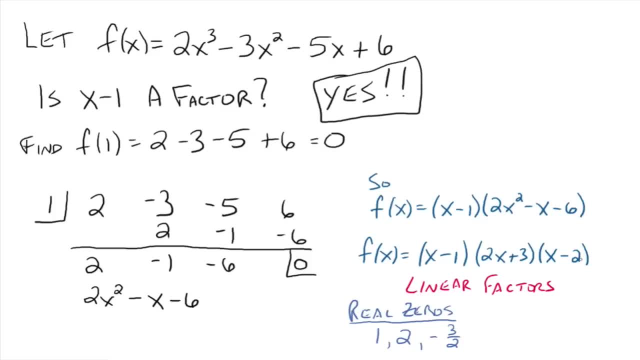 Does that make sense? Alright, so that's it on the remainder theorem and the factor theorem. So study well and please let me know if you have any questions.